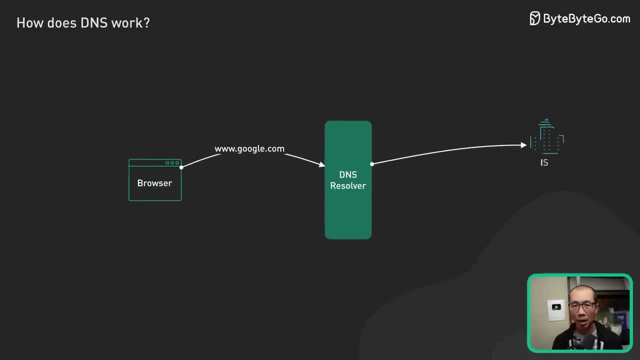 Now this DNS resolver could be from an ISP or from popular DNS providers like Cloudflare's 1.1.1.1, or Google's 8.8.8.8.. If the DNS resolver does not have the answer in its 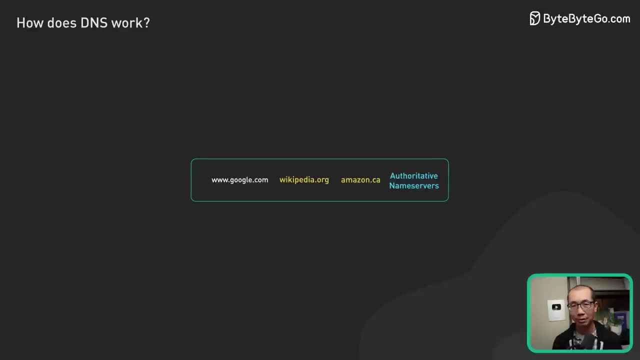 it finds the right authoritative nameserver and asks it: The authoritative nameserver is the one that holds the answer. When we update a domain's DNS records, as a site owner we are updating its authoritative nameserver. How does the DNS resolver find the authoritative nameserver? This is where the system of DNS 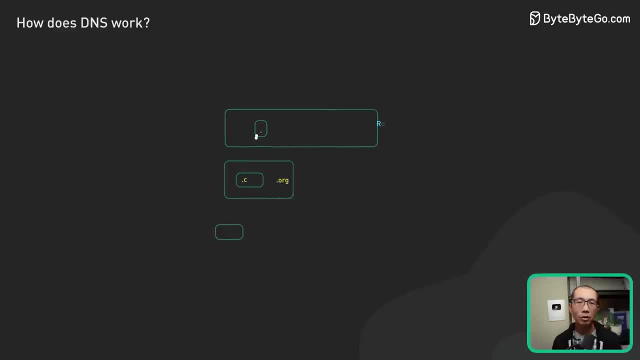 gets interesting. There are three main levels of authoritative DNS servers. They are the root nameserver, the top-level domain or TLD nameservers, and the authoritative nameservers for the domains. The root nameservers store the IP addresses of the TLD nameservers. There are 13 logical root nameservers. Each root nameserver has a single IP address assigned to it. There are actually many physical servers behind each IP address. Through the magic of Anycast, we get routed to the one closest to us. 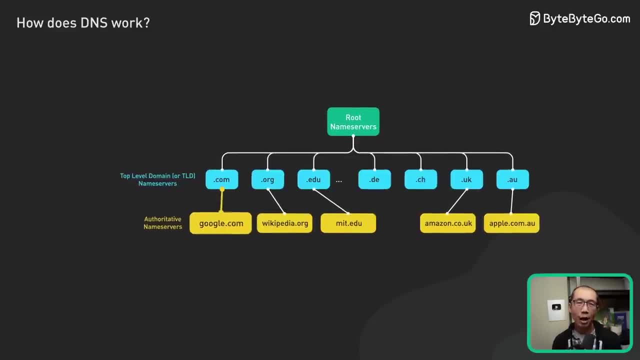 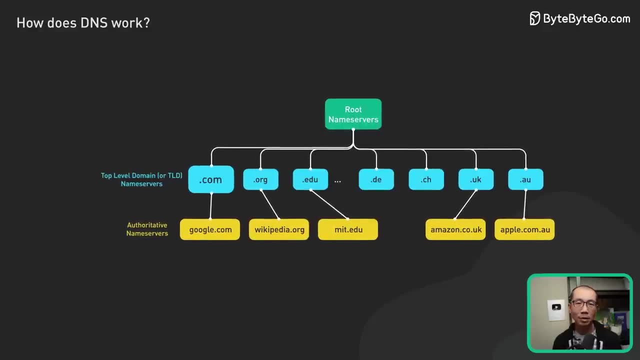 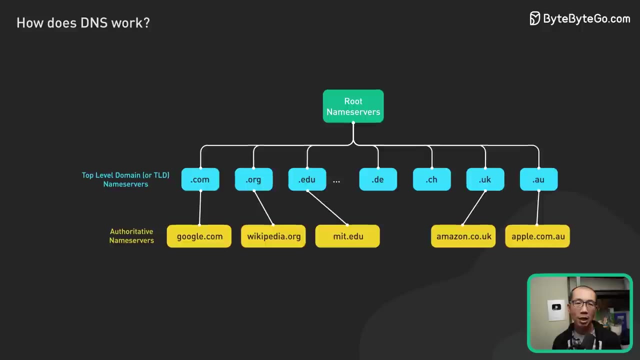 The TLD nameservers store the IP addresses of the authoritative nameservers for all the domains under them. There are many types of TLD names. We are all familiar with com, org and edu. There are also country code TLDs like de and uk. There are many others. 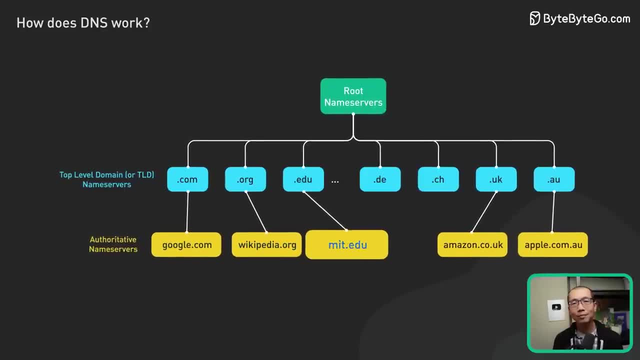 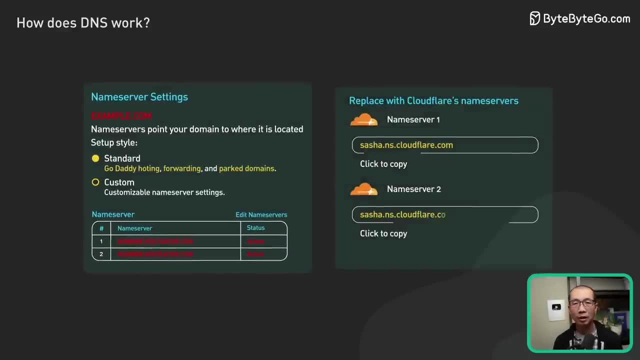 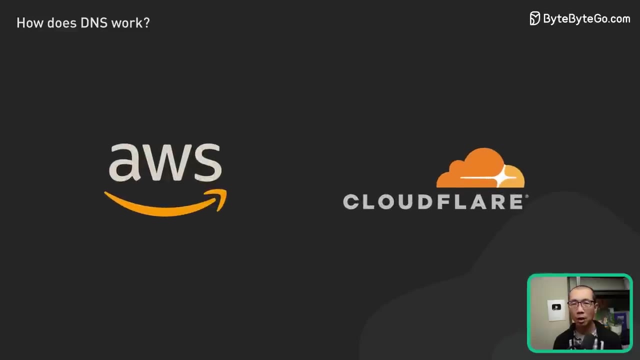 The authoritative nameservers for a domain provide well authoritative answers to DNS queries. When we register a domain, we can see that the domain has an authoritative nameserver. When we register a domain, the registrar hosts the authoritative nameservers by default, but we can change them to others- Cloud providers like AWS and Cloudflare. 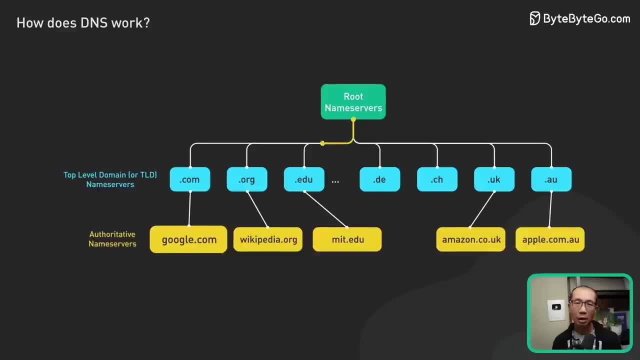 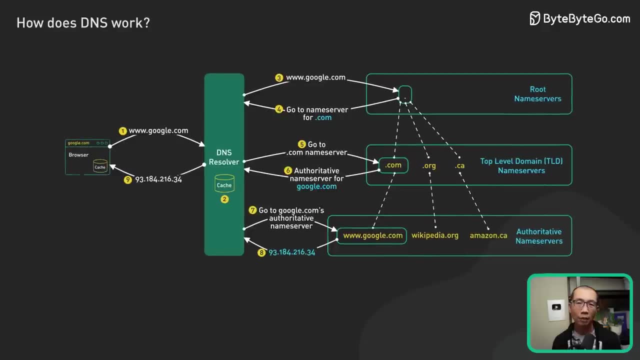 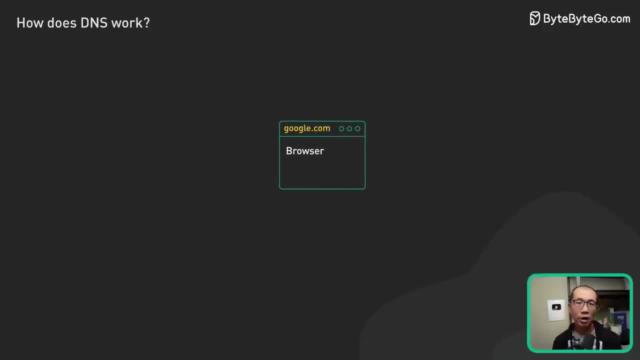 run robust authoritative nameservers. This hierarchical design makes DNS highly decentralized and robust. Now let's walk through the life of a typical DNS query. The user types googlecom into the browser. The browser first checks its cache. If it has no answer, it makes an operating system call to try to get the answer. 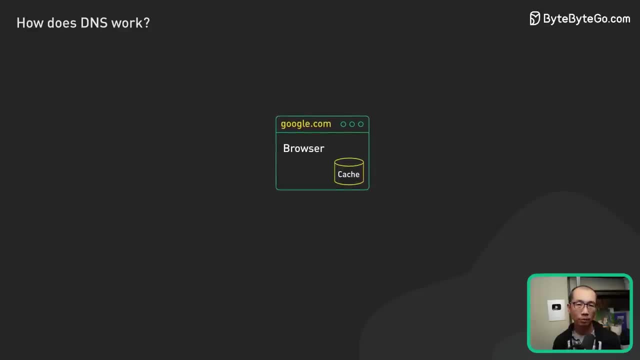 The operating system call would most likely have its own cache too. If the answer isn't there, it reaches out to the DNS resolver. The DNS resolver first checks its cache. If it is not there or if the answer has expired, it asks the root nameserver. The root nameserver responds. 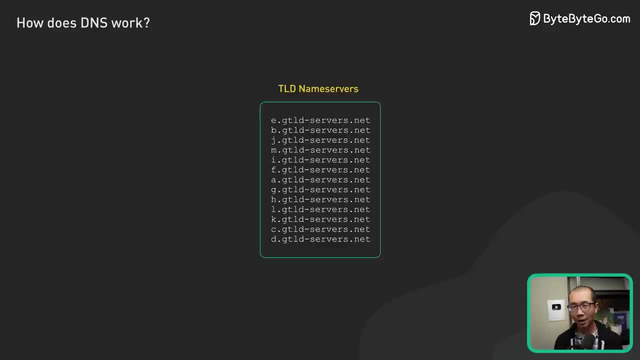 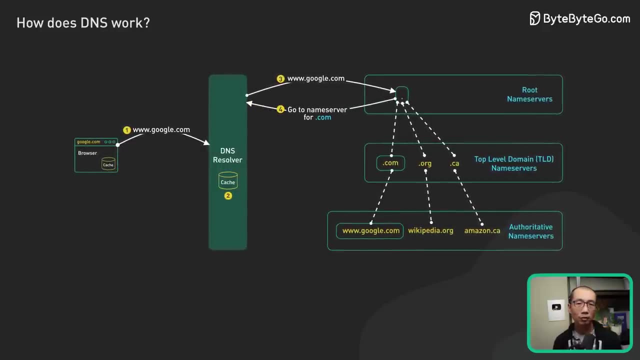 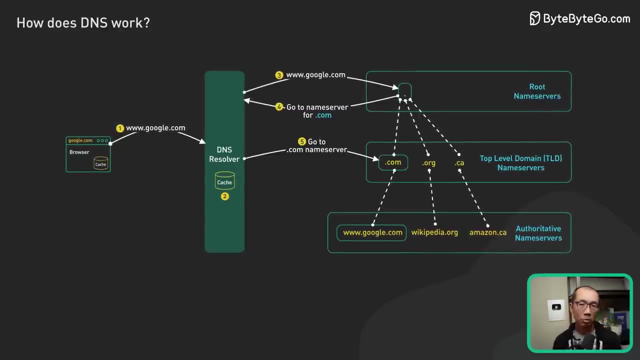 with the list of the com TLD nameservers. Note that since com is such a common TLD, the resolver most likely already caches the IP addresses for those com TLD nameservers. The DNS resolver then reaches out to the com TLD nameserver and the com TLD nameserver returns.